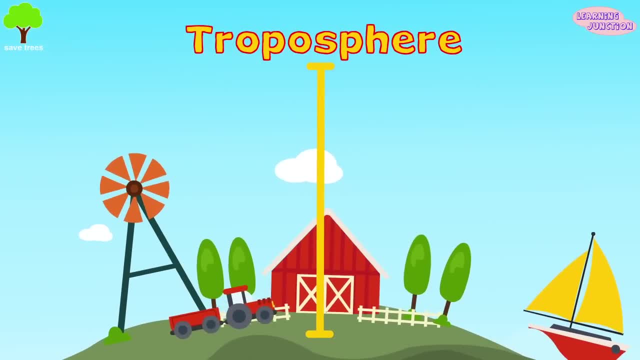 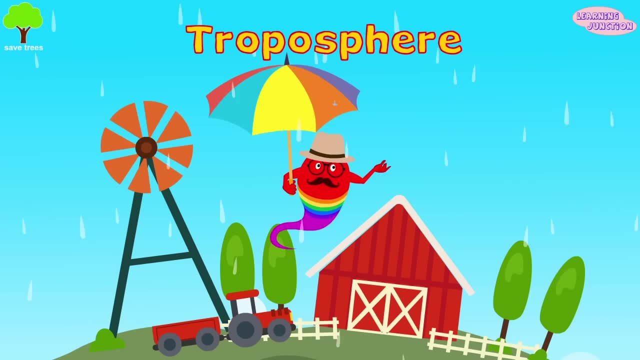 It's also the one where we all live in. It extends from the Earth's surface to about 12.5 miles in the sky. Our weather is formed in the sphere. Water evaporates. Water evaporates from land to become snow or rain. 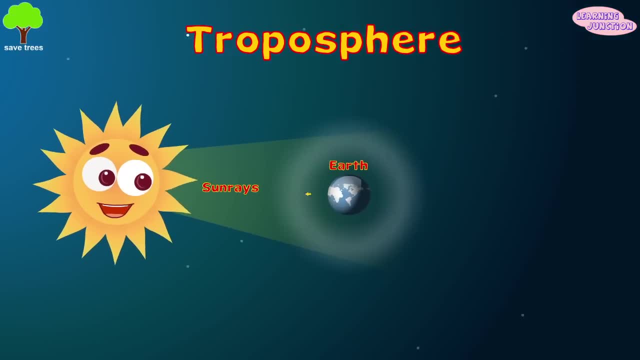 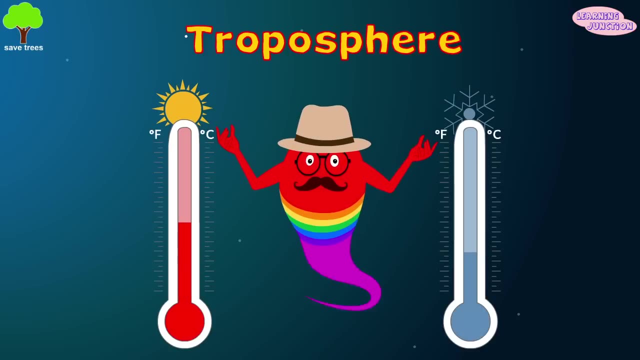 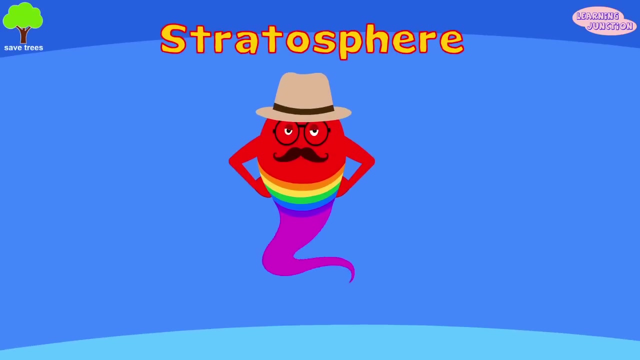 The vapor contributes to the greenhouse effect. It traps the sun's heat close to our planet. As a result, warm or cool weather comes. Hot air balloons fly in this layer, The stratosphere. The layer above the troposphere is called the stratosphere. 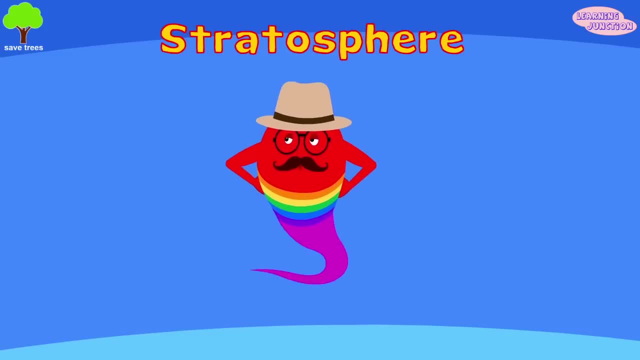 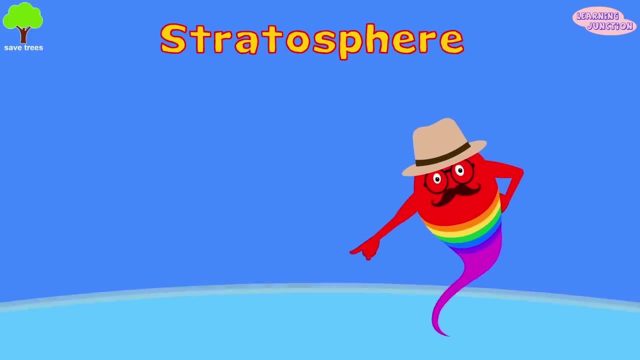 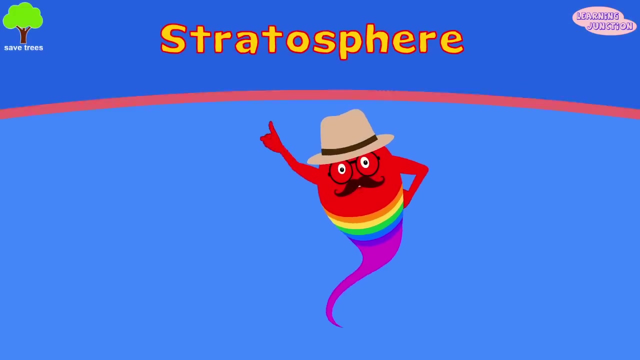 Stratosphere spans from the tropopause to about 31 miles up, containing about 20% of the Earth's gas. The ozone layer is found in this sphere, which protects us from harmful rays from the sun. The top part of the stratosphere is the hottest because the ozone layer generates a lot of heat. 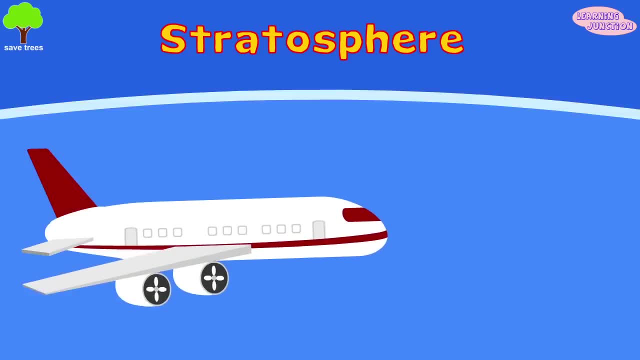 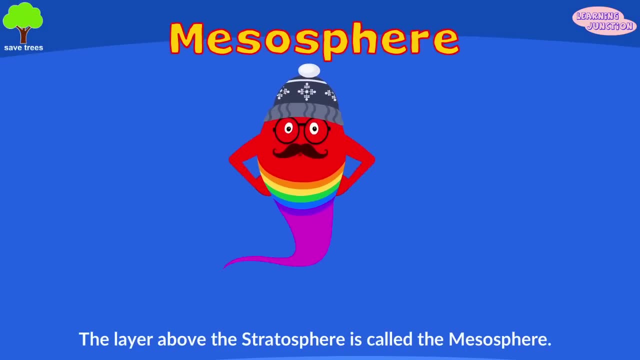 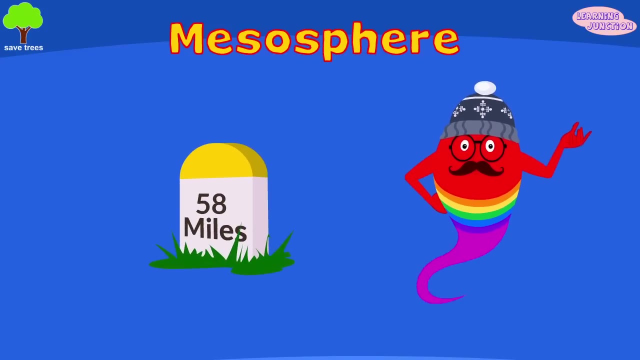 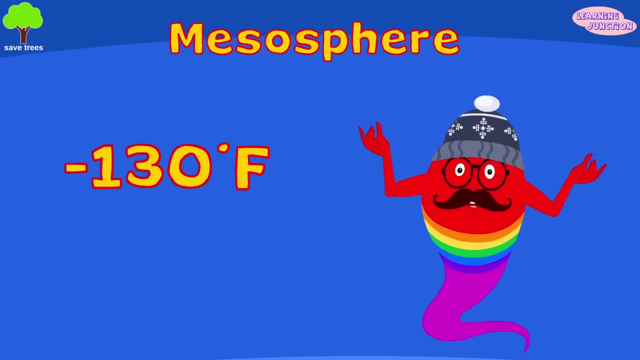 Airplanes and the jet aircraft fly in the stratosphere layer. Mesosphere- The next atmospheric layer is known as the mesosphere. It extends from the stratosphere to approximately 58 miles high. It is the coldest layer of atmosphere, about minus 130 degrees Fahrenheit near the top. 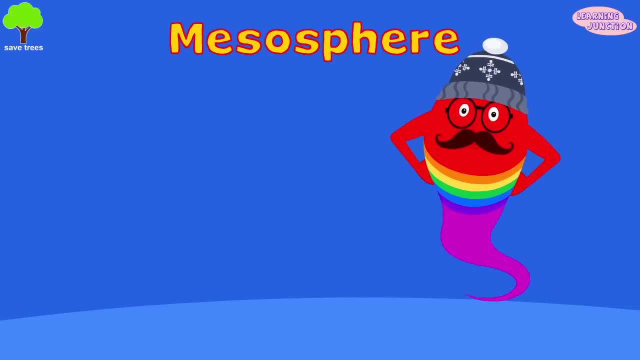 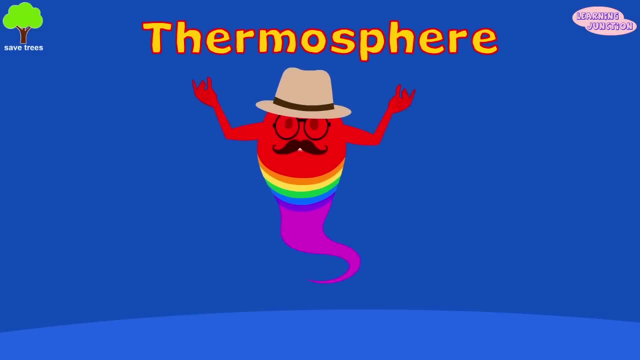 This is the part where most meteors burn up, Sounding rockets and others may go up to the mesosphere Thermosphere. It is the layer above the mesosphere. This layer spans almost 300 miles. It's very hot, as temperatures can reach up to 5,000 degrees Fahrenheit. 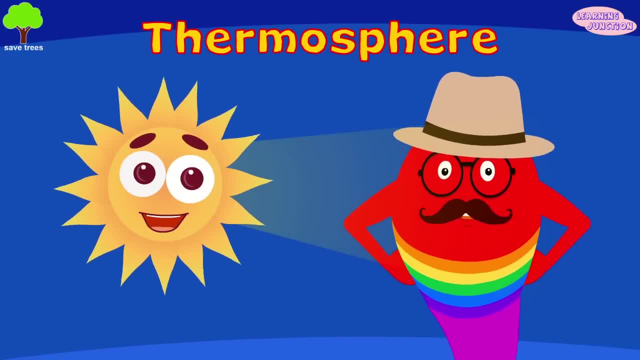 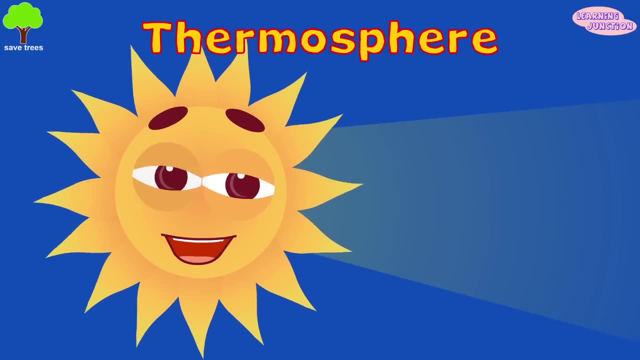 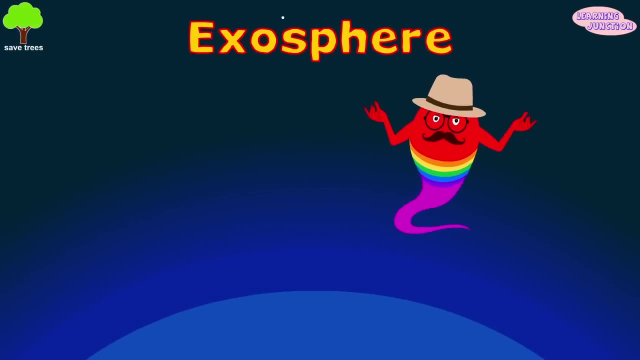 This is because the air in the thermosphere consumes lots of solar radiation. Most of the X-ray and UV radiations from the sun are absorbed in this sphere- Exosphere- It is the last layer of the stratosphere. The exosphere starts at the thermosphere, but it doesn't really have a sharp end.